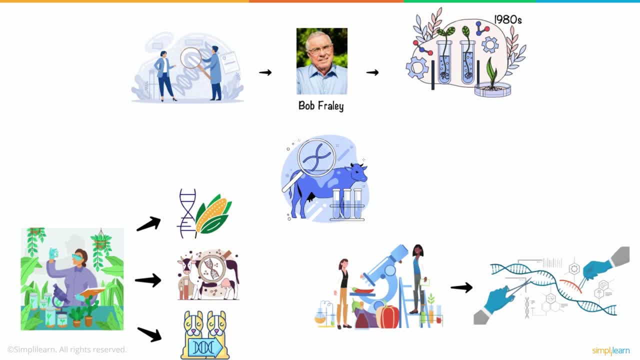 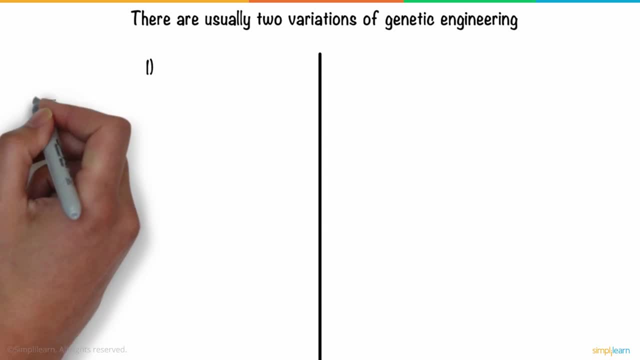 for researchers to directly alter the DNA of animals, plants and microbes. There are usually two variations of genetic engineering. The first variant has the original DNA structure of an organism fused with some foreign genes to introduce newer characteristics or features in the resultant GMO. For example, plant genes are often used with certain germicidal. 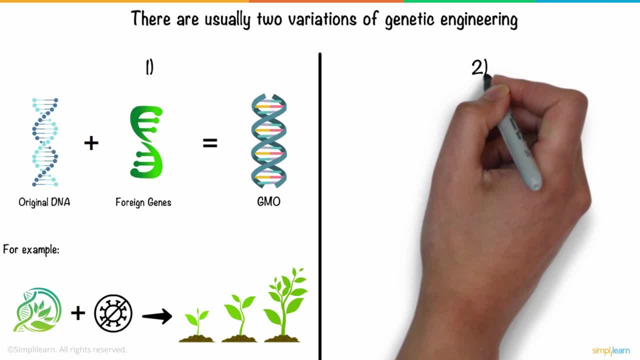 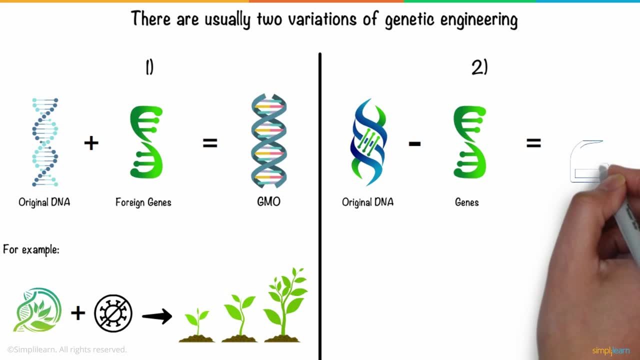 cells to facilitate long-term growth. The second type features the removal of certain genes from a DNA structure to eliminate the gene structure. For example, the DNA structure of a plant is used to eliminate certain behavior or characteristics that may be unwanted in the GMO. 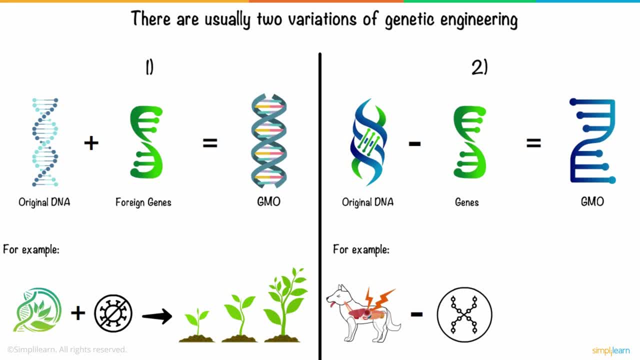 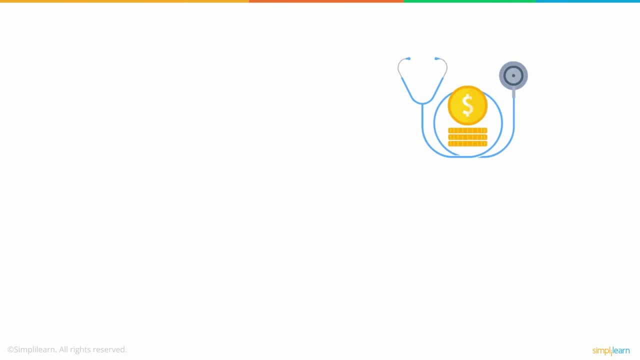 For example, removing a particular gene or enzyme from a species reduces its chances of falling prey to cancerous tumors. With so much investment in digital Scientology, scientists don't have to create thousands of experiments and store them physically. Experiments on genome structures are further accelerated and easier to mass-propagate, since 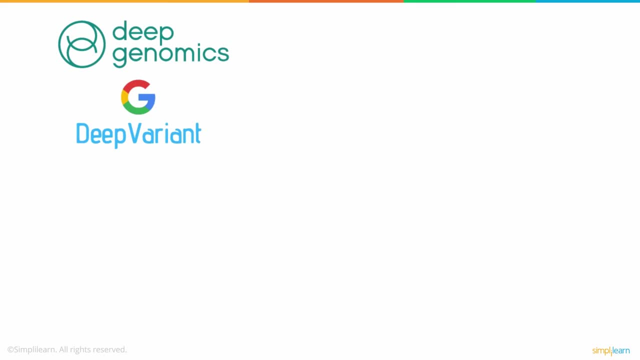 the advent of machine learning and artificial learning. Organizations like Google's Deep Variant and Deep Genomics have machine learning models to facilitate easier drug tests and gene sequencing projects. Another institution, Sophia Genetics, has made progress using AI models to prescribe personalized medications for cancer patients and other diseases. 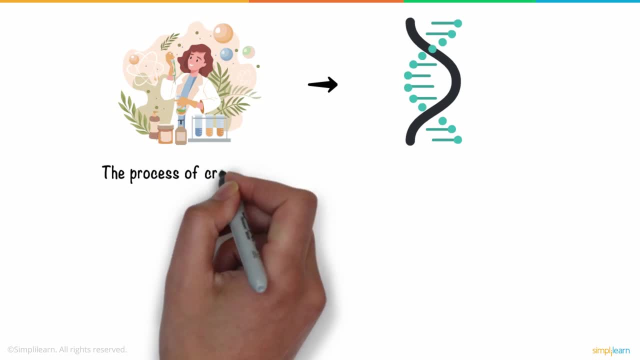 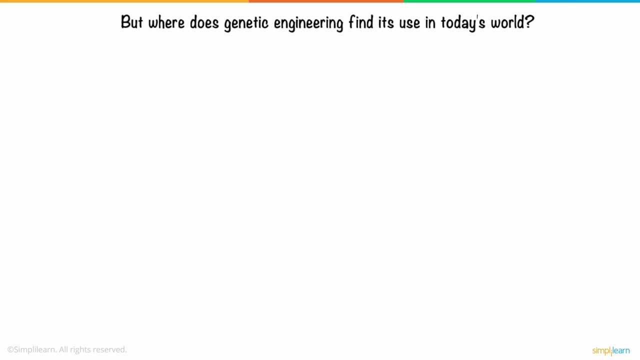 Scientists have also been able to perform gene cloning, which is essentially the process of creating an exact duplicate of base DNA material. This is especially helpful in medical fields, where gene cloning can accelerate the rapid testing of vaccines and serums. But where does genetic engineering find its use in today's world? 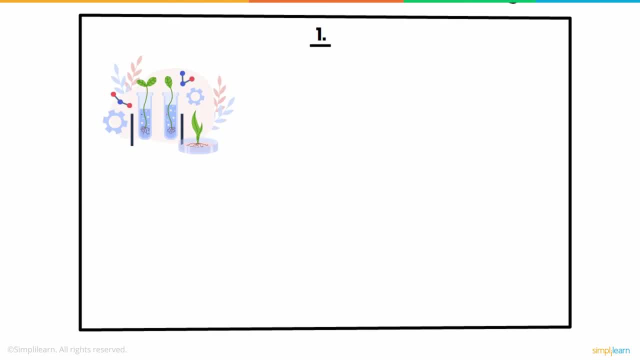 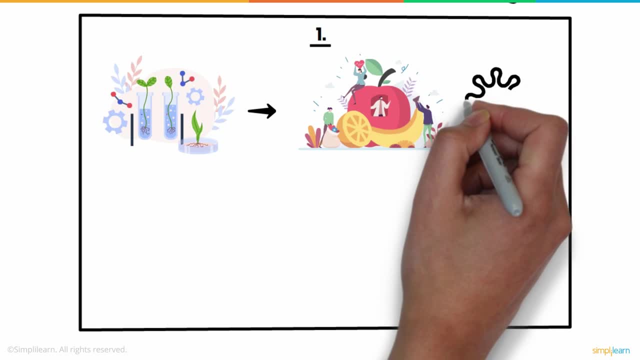 1. Genetic engineering technology is widely used to modify crop plants' genotypes to increase their productivity, nutritional value, protein content, resistance to disease and fertilizer usage. High-yielding grain pulse and vegetable crops can be produced using recombinant DNA. 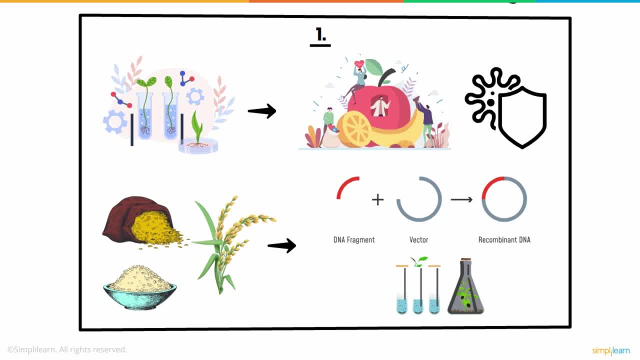 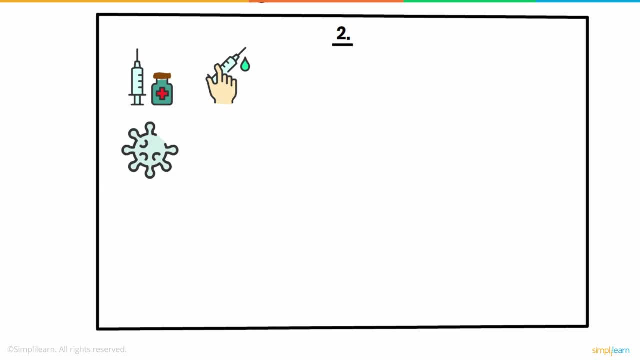 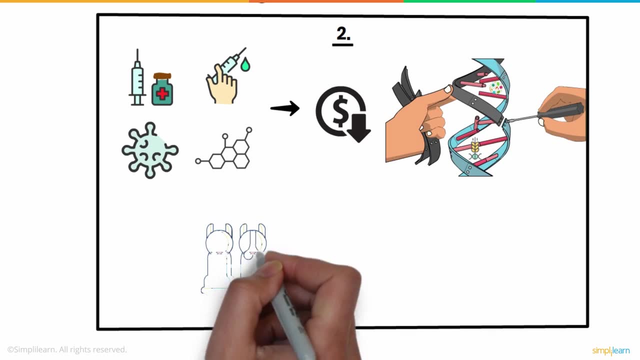 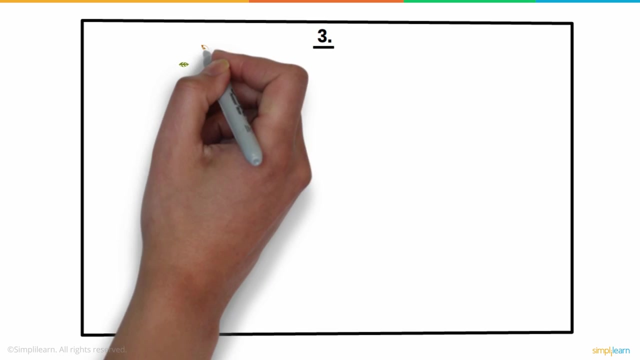 2. It is possible to generate large quantities of important medications, vaccines, enzymes and hormones at minimal cost by manipulating microorganisms and plant-based materials. Vaccines created with gene cloning technology do not possess any contaminants and are completely safe. 3.